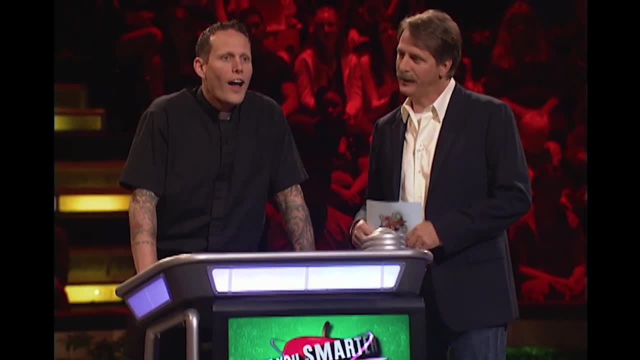 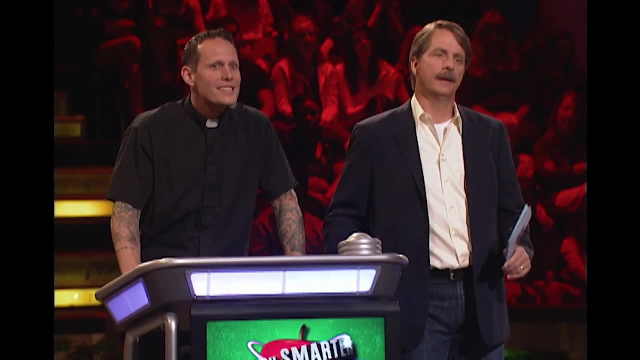 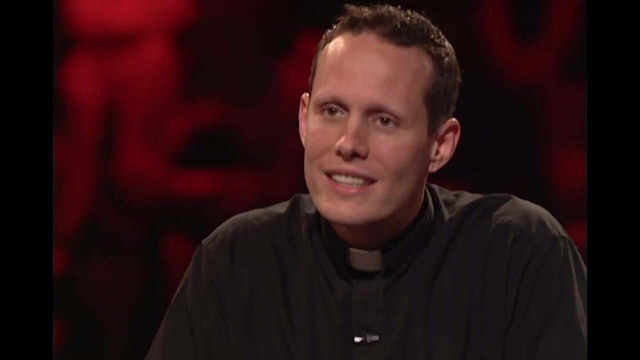 TJ has locked in his answer. What are you thinking, Henry? I'm thinking- I don't even know that word- A sesquicentennial is 100.. OK, But that's not the question at all. Oh, I've got some cheats left and I think. 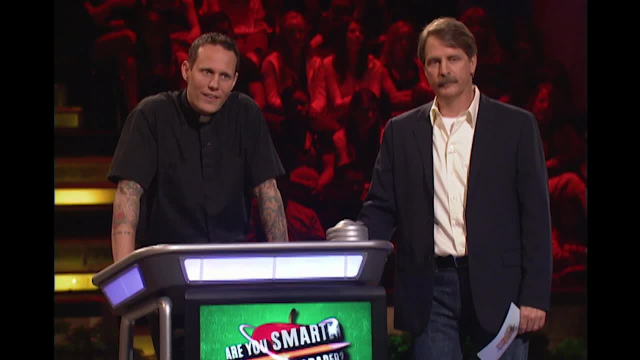 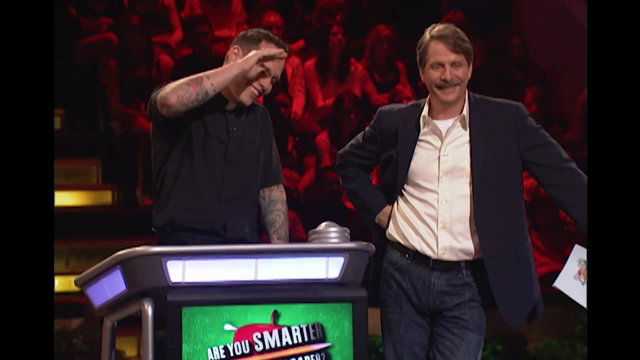 I'm going to have to go to those. You know what? I'm going to have to go the copy, because if I peek I'm going to take it anyway, because I am clueless. I am going to go the copy. 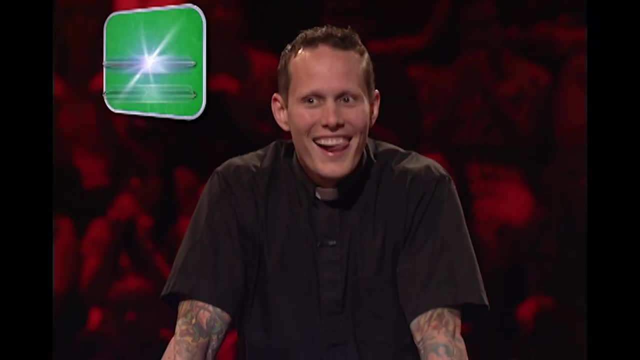 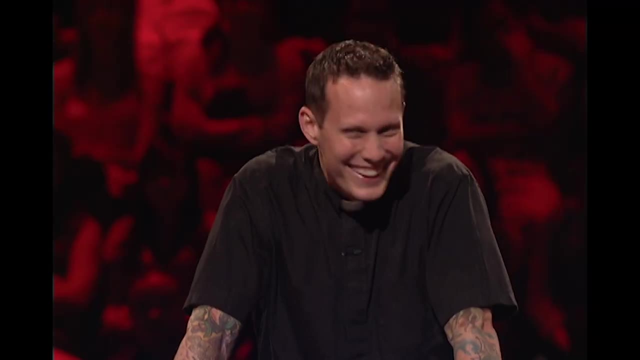 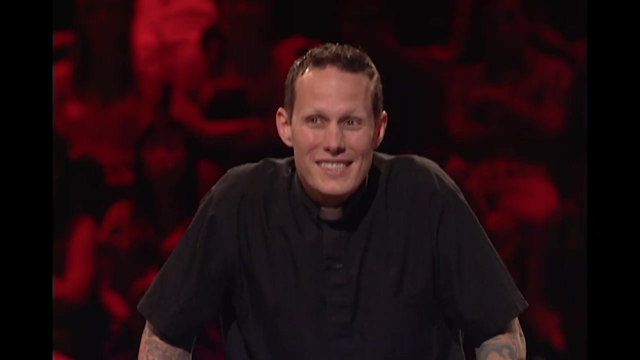 Oh, I hope you're good, TJ. Oh, I hope you're good. It's what the world needs. is a clueless pastor, Sesquicentennial. What would you have guessed if he hadn't been here? Ses sounds like six, maybe, or seven. 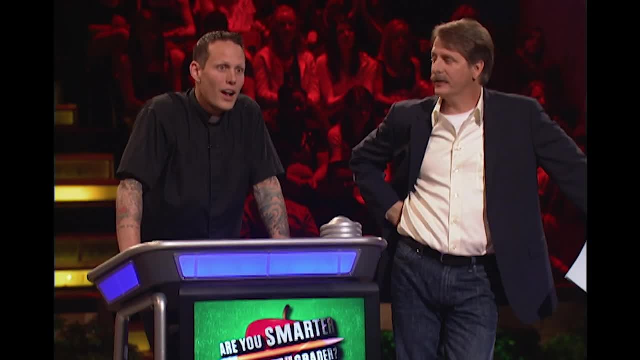 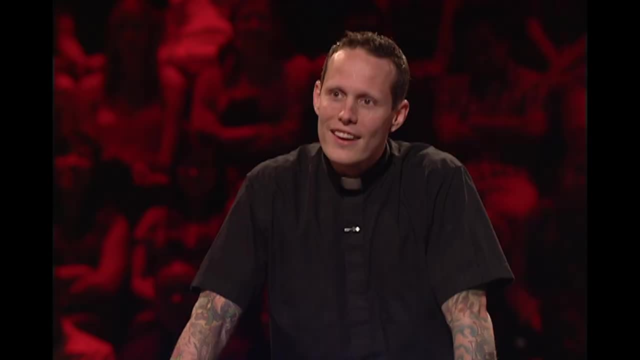 700 years. 700 is actually absolutely wrong. OK, good, Good, It's not even close. So I would have been absolutely wrong. You would have been absolutely wrong. I have no clue. I don't even know that word. 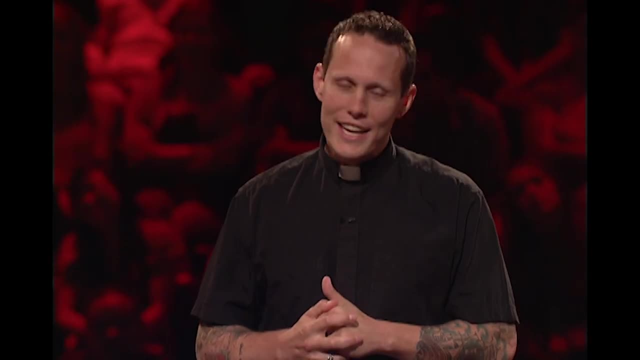 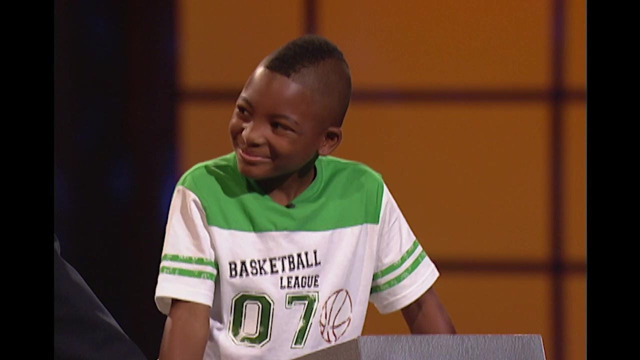 But I bet you this: I bet for the rest of your life you'll remember what it means. I guarantee that And I'm hoping TJ learned that this year. I'm really, really hoping he learned that this year. Sesqui means one and a half. 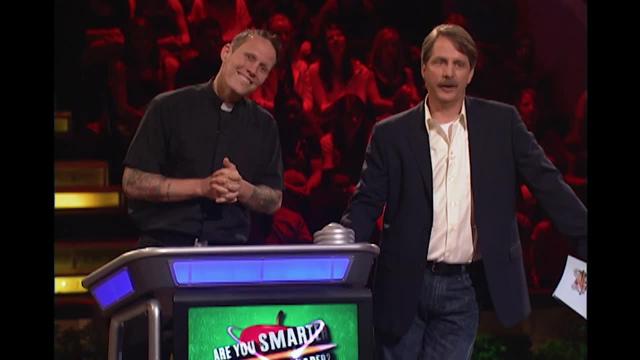 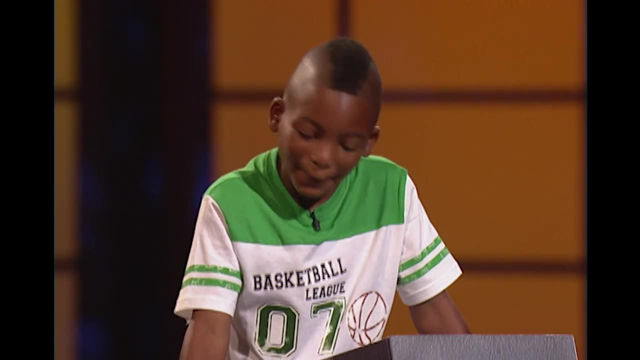 So it's 150 years. It is exactly 150 years. Oh, I'm hoping TJ knew that. If TJ said 150 years, you've got $12,500.. If he said anything else, we're back to zero. Back to zero. 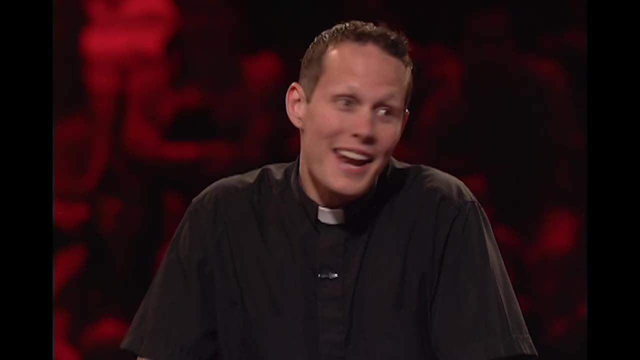 And I'm sure you're very big on forgiveness, right, I am. Hey, I didn't know it, But you know what I'm not going to have to? He's going to know it. Take a look at the board. 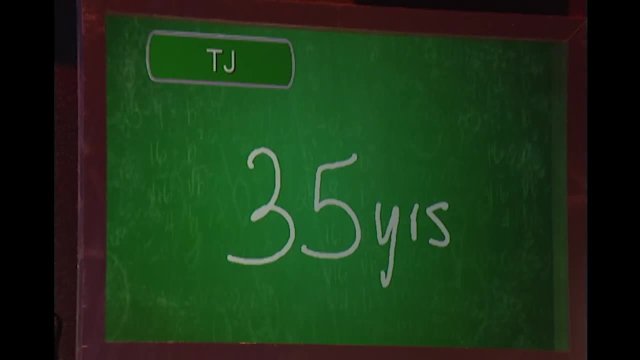 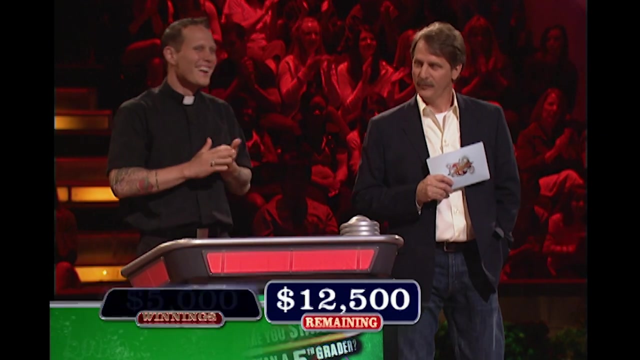 Your 10-year-old classmate said 35 years. Hey, that's OK, man, That's OK. I had no clue either. We'll get the money back Next time. Next time, You know it, We'll get it back. 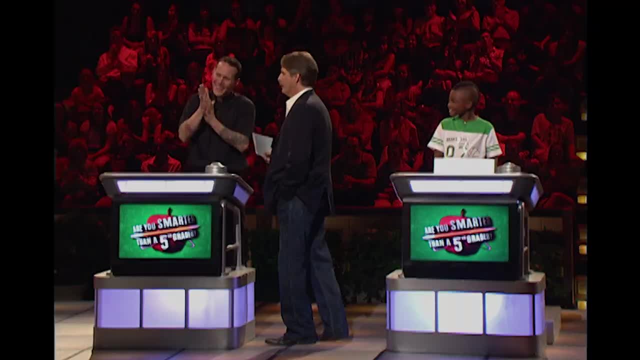 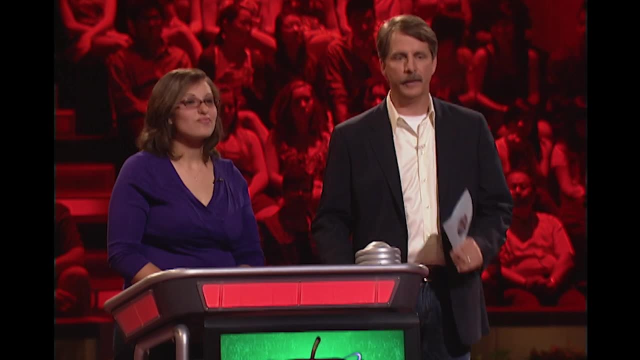 We'll get the money back. Woo, I like your attitude. OK, This one's ours. Chuck Yeager was the first American pilot to break the speed of sound barrier, not the first one to cross the Atlantic. OK, we've still got a lot of money up there. 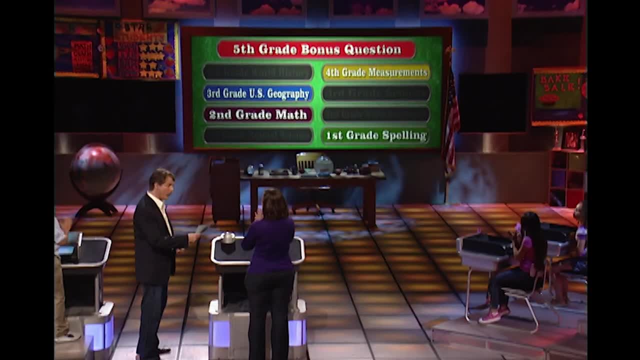 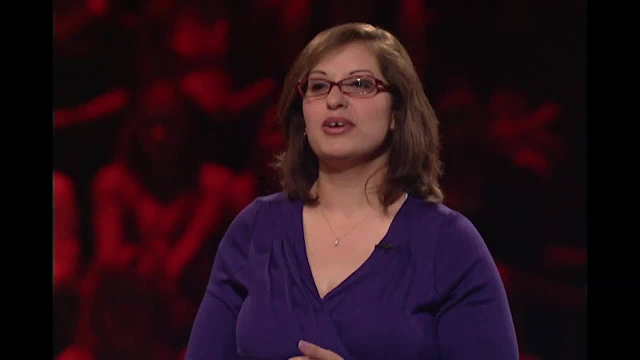 $12,500.. Four subjects remain. What would you like next? Measurement, Measurement, Measurement. OK, Our mind is good at measurement. OK, So I'm going to do measurements, Your fourth grade measurements. OK, This one's worth $7,500. Here is the question: The amount of energy needed to raise the temperature of one pound of water one degree Fahrenheit is measured in BTUs. What three words do the letters BTU stand for? The amount of energy needed to raise the temperature of one pound of water one degree Fahrenheit? 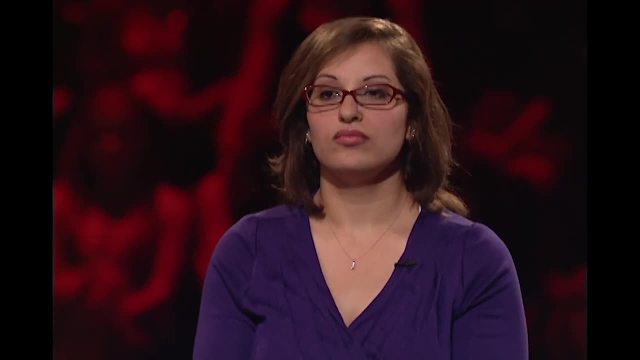 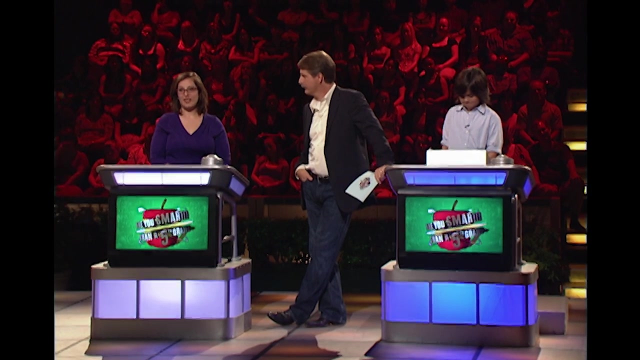 is measured in BTUs. What three words do the letters BTU stand for? The amount of energy needed to raise the temperature of one pound of water one degree Fahrenheit is measured in BTUs. Armand has locked in his answer. I don't want to use up my last cheat and 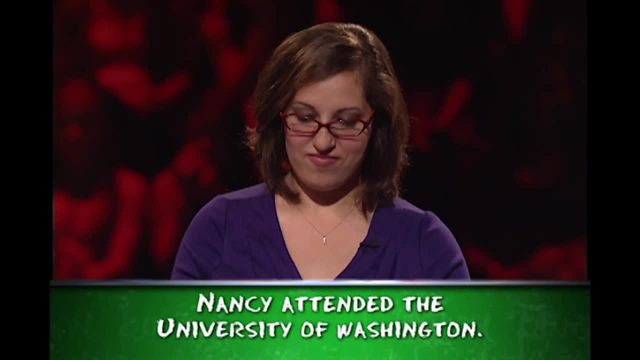 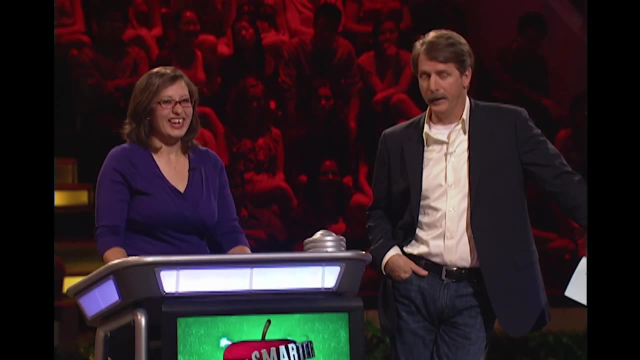 You know what? I think? I am going to use it. I think I am going to use it. No, no, I'm sorry. Can I be indecisive? Sure, You're a woman. yes, OK, I live in a house in the middle of the country. 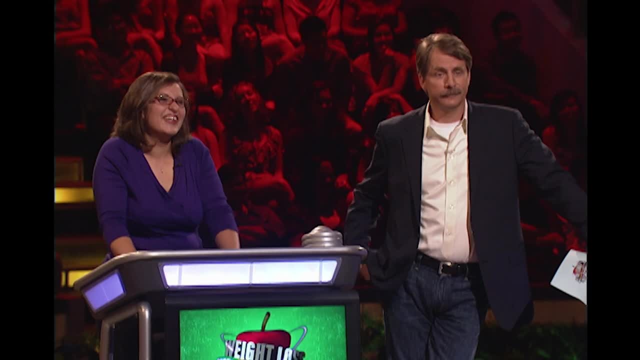 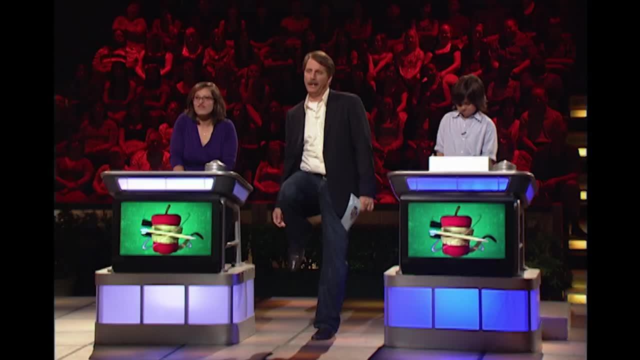 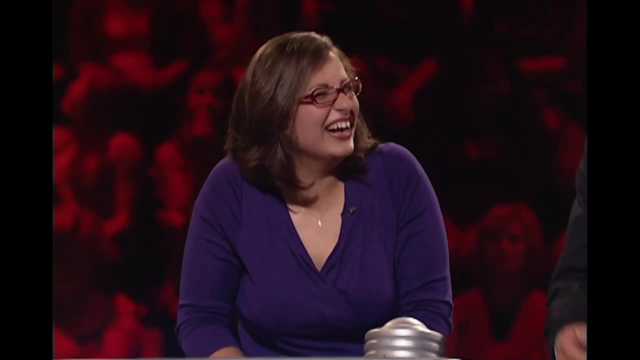 I should know, Honey, which shoes look better- These or these? She shouldn't ask you. I just mess with her. I'm like I don't know. Do it again, These or these? OK, What do you think? 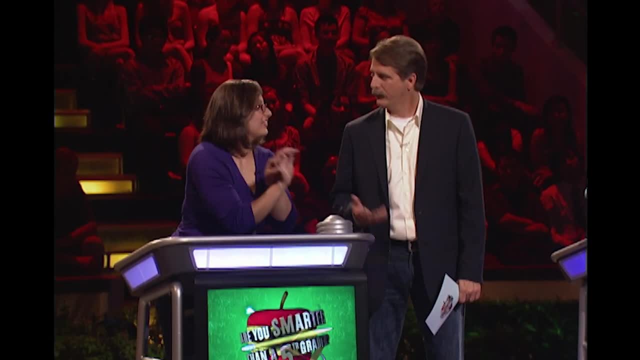 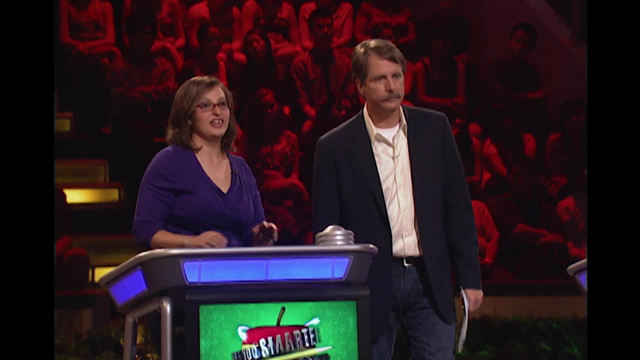 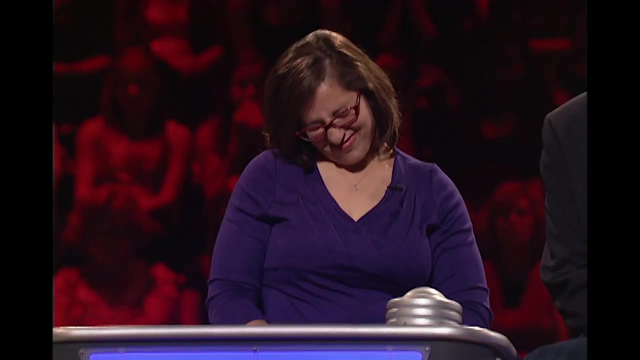 I think I'm just going to lock in a no answer. Can I do that? Throw something out there, Guess OK, BTU, BTU By the unit, By the unit, Locking it in All combustible materials measures, the BTUs. 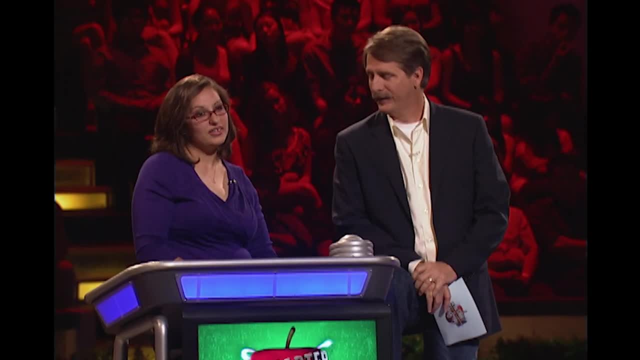 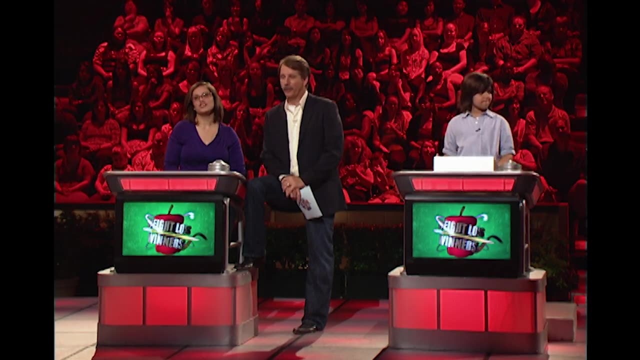 I can't believe you just guessed that. Is it really By the unit? Unit is correct By the is not. It is British thermal unit. British thermal unit, BTUs. I think we're going to go with fourth grade math. 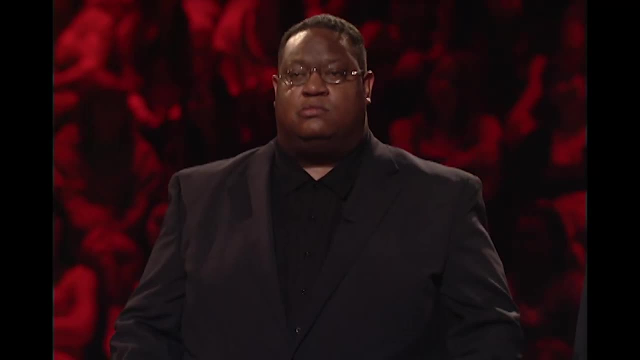 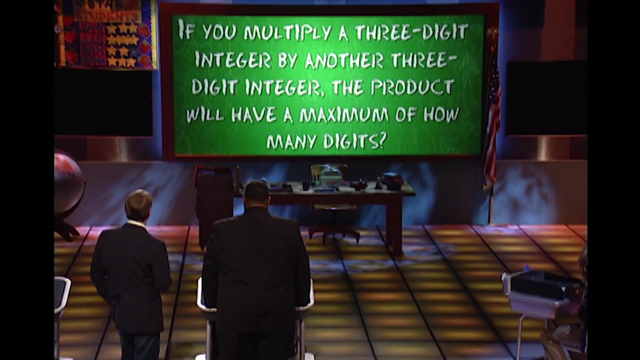 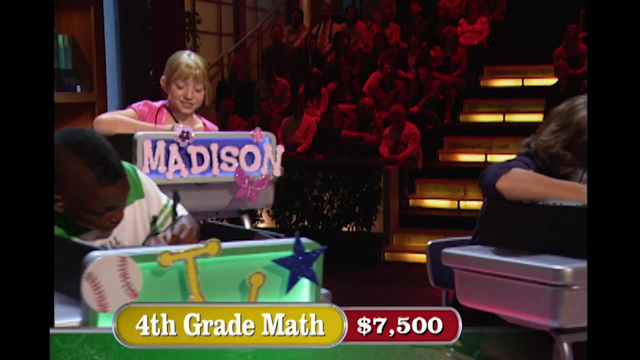 Fourth grade math. it is For $7,500.. Here is the fourth grade math question. If you multiply a three-digit integer by another three-digit integer, the product will have a maximum of how many digits? If you multiply a three-digit integer by another three-digit? 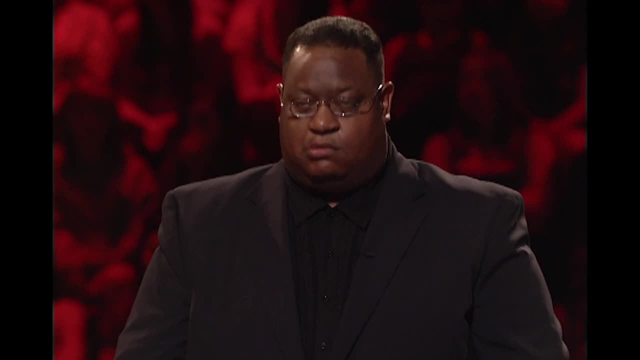 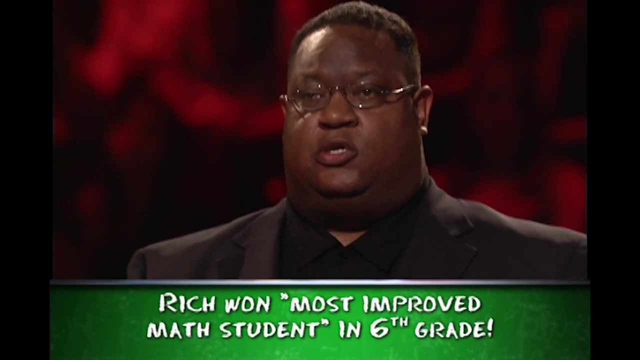 integer, the product will have a maximum of how many digits? OK, I believe that you will have a 1,, 2,, 3,, 4,, 5,, 6,, 7,, 8,, 9,, 10,. 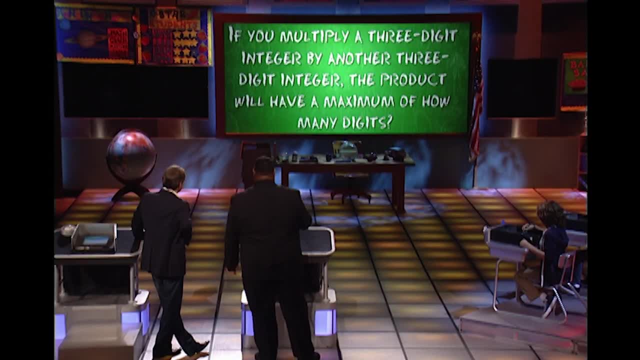 10,, 11,, 12,, 13,, 14,, 15,, 16,, 17,, 18,, 19,, 20,, 21,, 22,, 23,, 24,, 25,, 26,, 27,, 28,, 28,, 29,, 30,, 32,, 33,, 34,, 34,, 35,, 36,, 37,, 38,, 38,, 39,, 40,, 40,, 42,, 45,, 45,, 45,, 46,, 40,, 42,, 45,, 46,, 47,, 49,, 42,, 45,, 46,, 47,, 49,, 5,, 46,, 47,, 49,, 40,, 42,, 45,, 47,, 49,, 40,, 45,, 46,, 47,, 49,, 40,, 48,, 49,, 50,, 51,, 52,, 51,, 52,, 52,, 53,, 52,, 53,, 52,, 53,, 54,, 56,, 55,, 57,, 58,, 58,, 69,, 51,, 72,, 53,, 59,, 52,, 53,, 54,, 55,, 55,, 56,, 57,, 68,, 69,, 70,, 80,, 80. 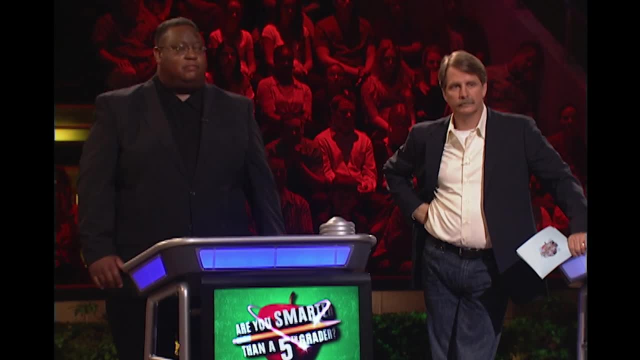 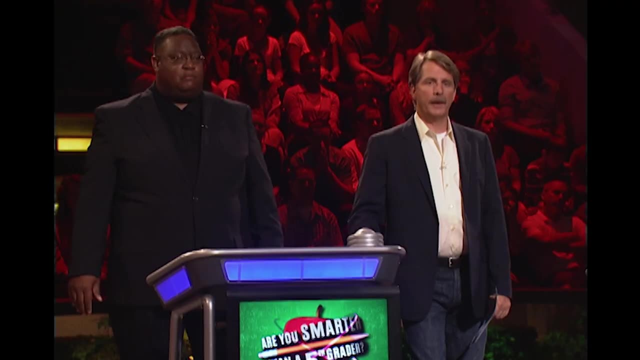 I believe you will have a five-digit number. I'm locking that in. Oh man, Let's see what happens here. If you multiply a three-digit integer by another three-digit integer, the product will have a maximum of how many digits. 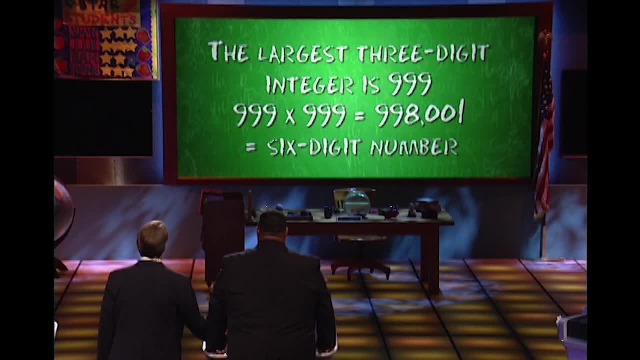 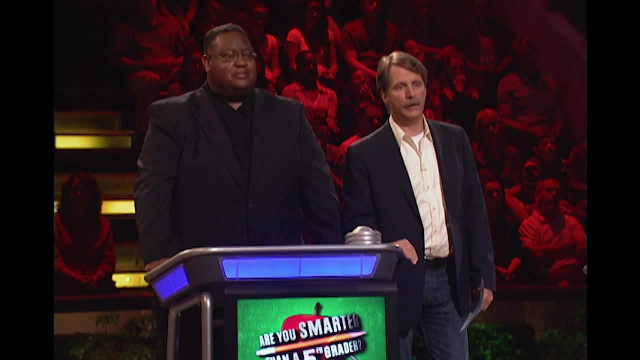 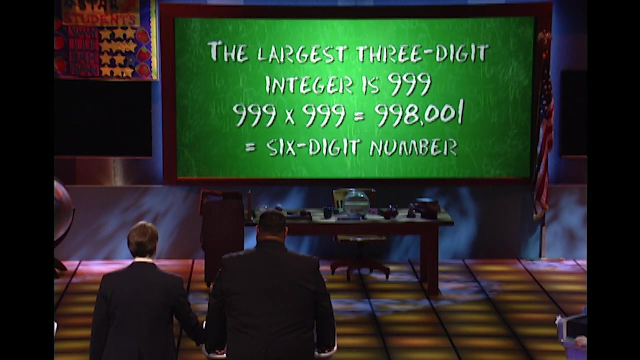 Let's take a look at the board. The largest three-digit integer is 999.. So if you multiplied 999 by 999, you would get 998,001, which is a six-digit number, And when you first did it out, you went 1,, 2,, 3,, 4,, 5,, 6.. 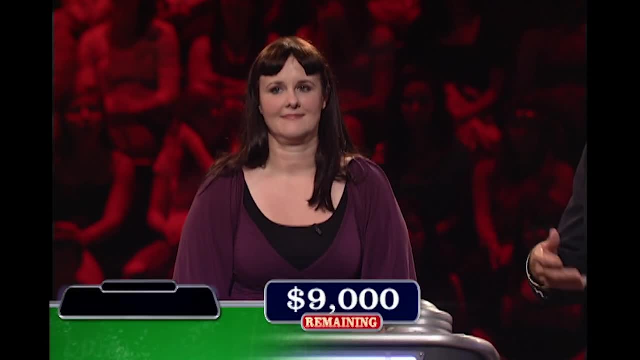 I sure did. Our contestant, Shelly Hartman, had a whole bunch of money and gave it back. but now we're on the comeback trail. We're not giving money back anymore, are we? I hope not. You got $3,500. 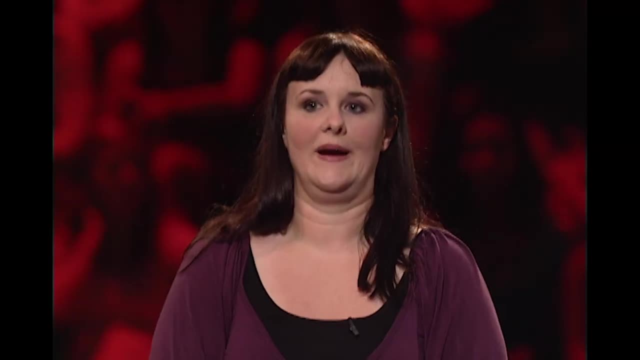 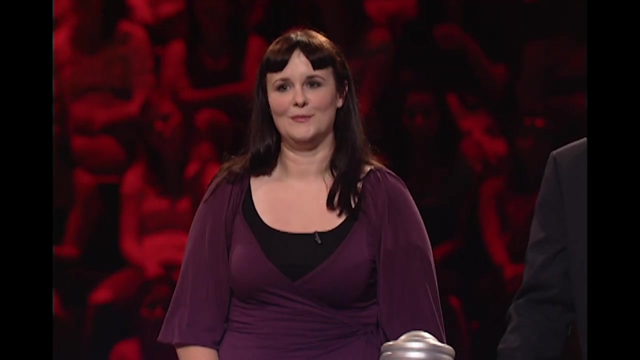 Three subjects remain. Shelly, I have to go with math. Got to get the math out of the way. Are you good at math? No, No, No. Be good at this one. I hope so For $7,500,. here's the math question. 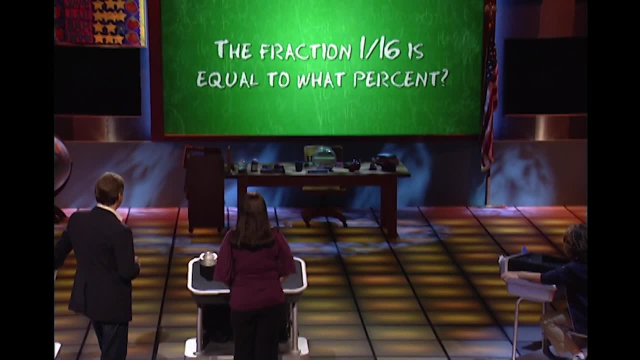 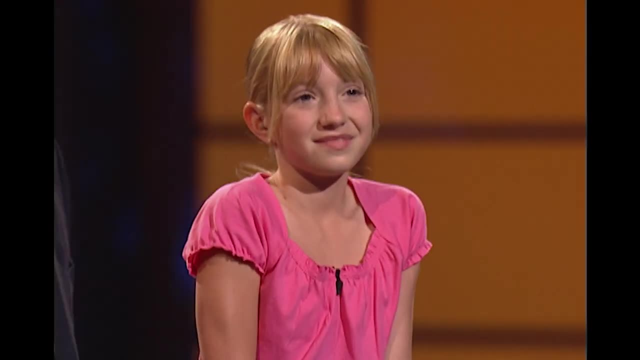 The fraction 1- 16th is equal to what percent? The fraction 1- 16th is equal to what percent? All right, Madison has locked in her answer. What are you thinking, Shelly? I hate math. That's what I'm thinking. Talk it out. Yeah, I was thinking 1 10th is 10%. 1 10th of 100 is 10%. So it seems like 1- 16th would be less than that, more like 6%, And that's what I'm thinking. 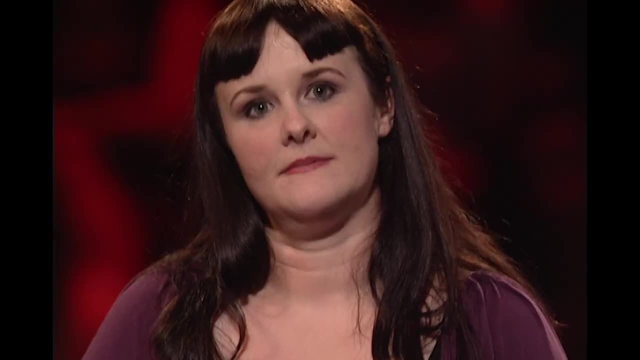 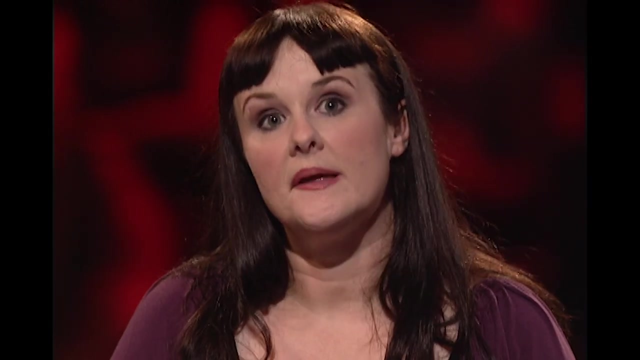 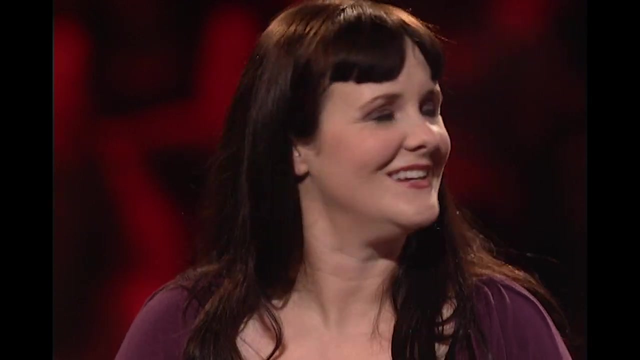 It makes sense that 16 would be 6%, 5% would be 1, 20th. So I think I'm just going to Go with my gut and hope I don't shoot myself later. So I'm going to go with 6%. 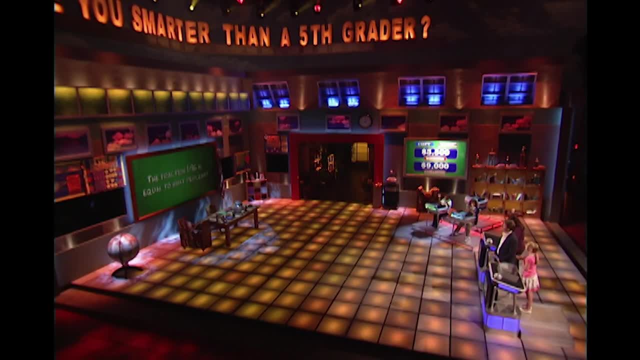 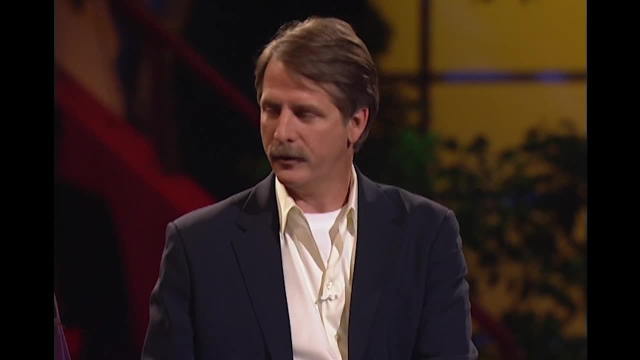 And we'll knock it in 6%. Whenever I see a fraction thing, I always go back to the thing in school about the pie. I imagine a piece of pie. So if you had a piece of pie cut four ways, that would be. A quarter, 25%, right, Mm-hmm, That's one-fourth of that is 25%. So if then you half the fourth, that would be one-eighth, And so instead of 25%, that's 12.5% right. 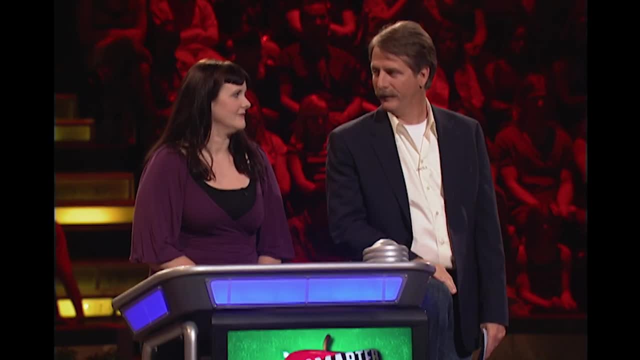 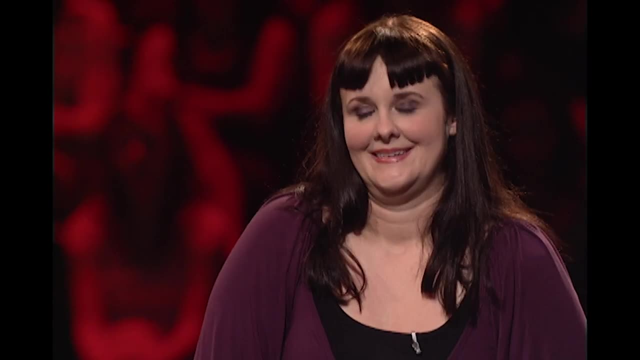 Right, And then if you half that again, instead of 12.5, you have 6.25.. Oh no, Take a look at the board. 1: 16th equals 0.625.. 6.25%. 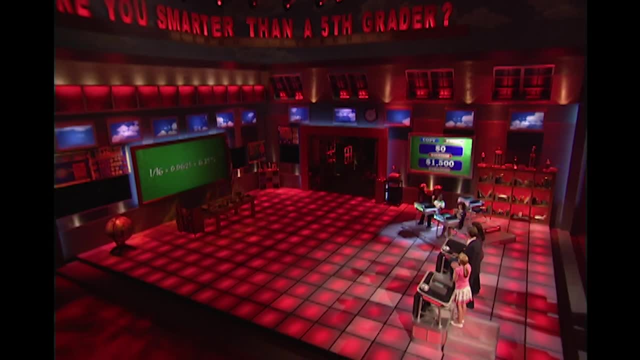 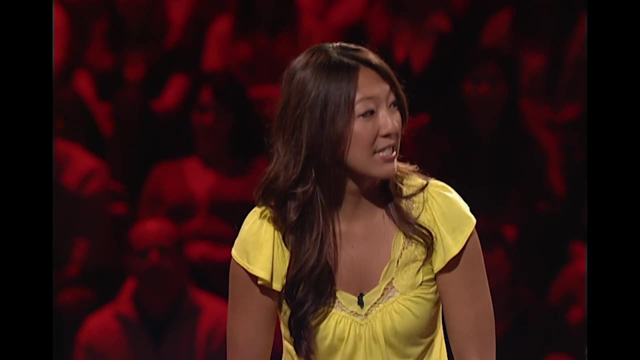 So close, Yeah, So close. We've got TJ out of the subjects on the board. what do you like the best? Math, Math, Oh, let's do it. TJ, Let's go- fourth grade math. 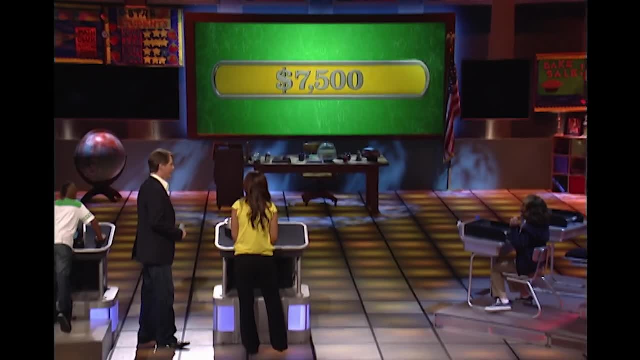 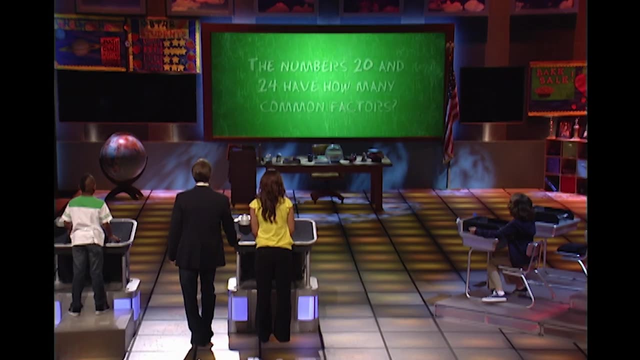 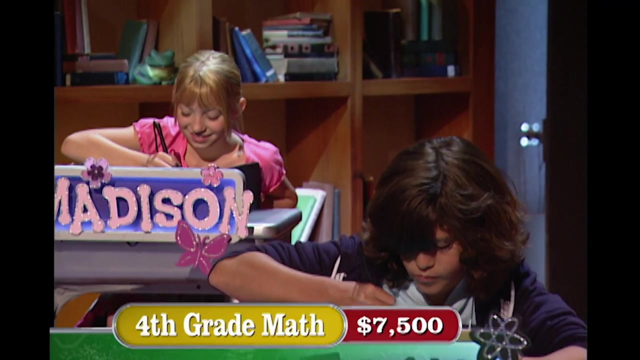 Fourth grade math. Going to the top: Go fourth grade math, Get it right, you'll have $12,500.. The fourth grade math question is: The numbers 20 and 24 have how many common factors? The numbers 20 and 24 have how many common factors? 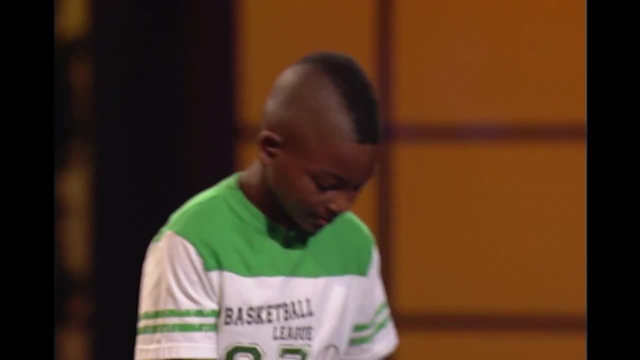 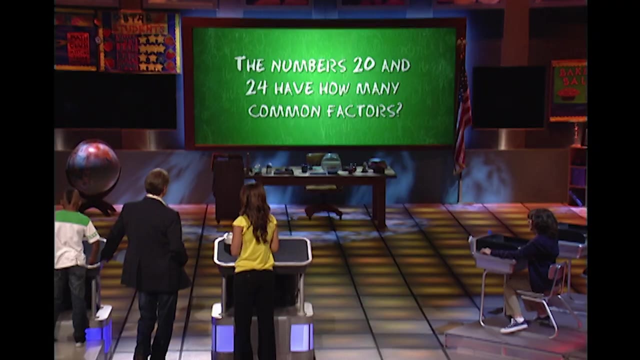 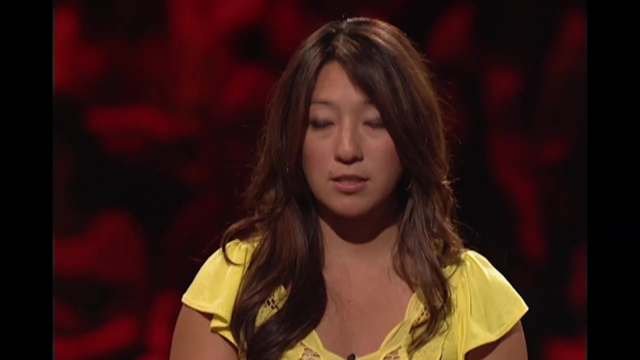 All right, TJ has locked in his answer. Common factors. I know it's a multiple of a number. I know they both have the common factor of 2.. They both have the common factor of 4.. Now I think that 1 would be considered a common factor. 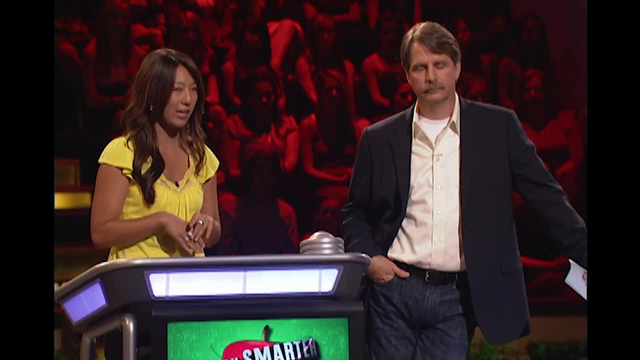 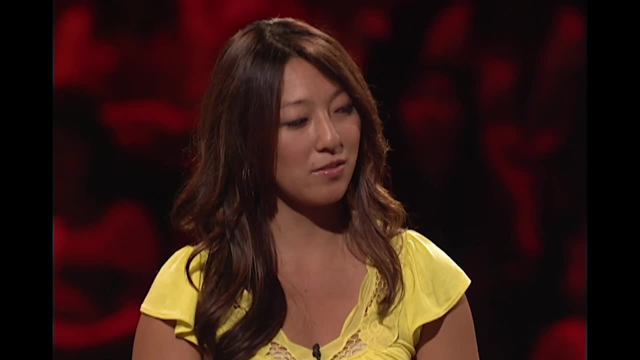 1. 1. 1. 1.. I'm gonna take a peek at TJ's answer over there. Okay, peek means you can look at their answer. If you like it, you can go with it, If not, you can go with something else. 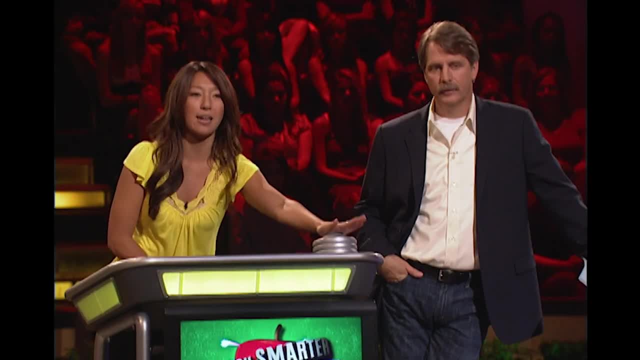 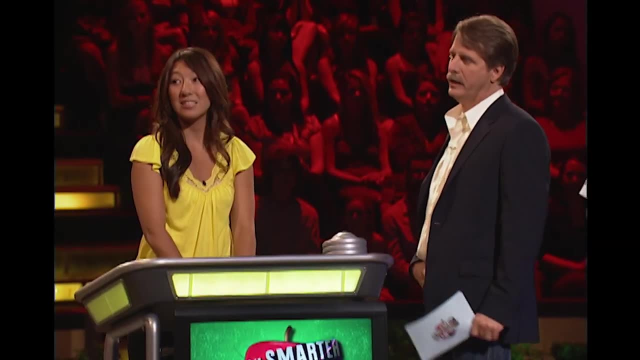 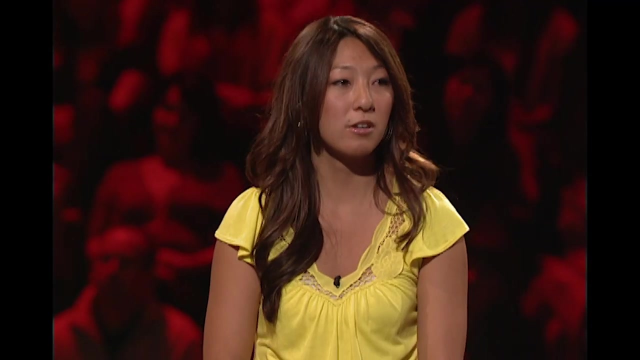 Two, one, two. I'm gonna peek, Peek. Yes, The numbers 20 and 24 have how many common factors. Take a look at the board. TJ said one One Man. He really broke that down Um one, four, two.